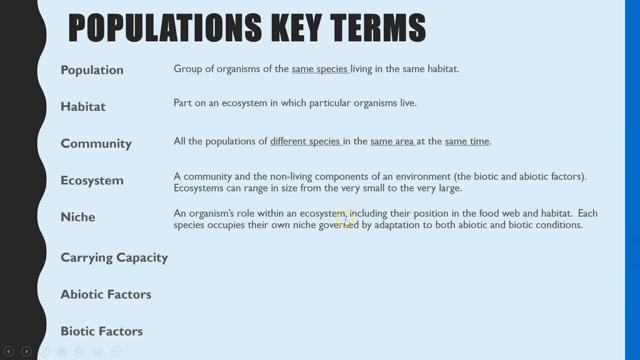 element. it's their role within the ecosystem. We have to point out some examples of what we mean by their role. So, for example, their position in the food web, So what they eat and what eats them and their habitat And each species. now, this second part isn't part of the definition, it's just a fact. each species. 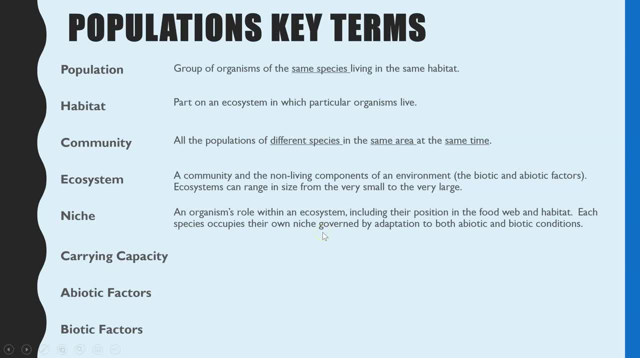 occupies their own niche. So no two species can share a niche. If two species start to try and share a niche, meaning their position in the food web and habitat, then they will go into competition with each other and one species will get out-competed to make sure only one species can exist in one niche. 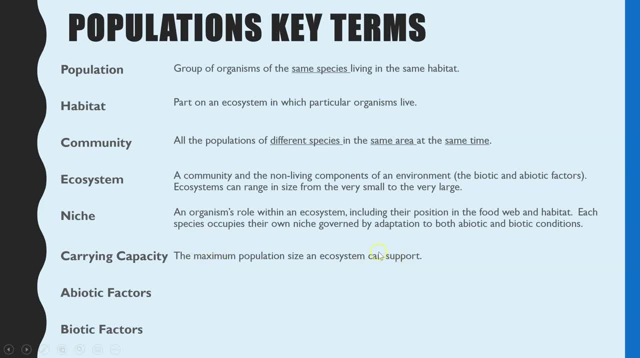 Carrying capacity is the maximum population size an ecosystem can hold, And when a population reaches that carrying capacity, if the population size does increase, what you'll then find is that population will have an increased death rate to bring it back down to the carrying capacity, And that might be. 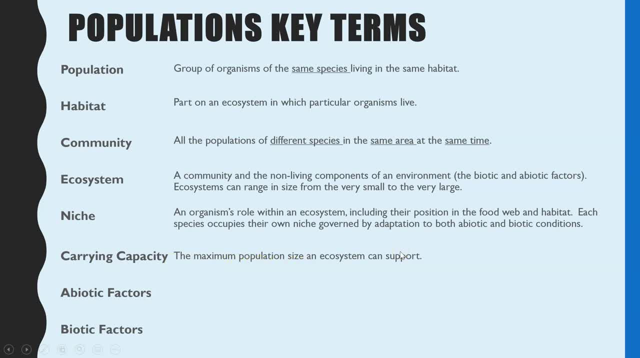 because there's now not enough food in the ecosystem to support all the individuals, Or it might be that there's not enough space or enough of the habitat. Abiotic factors are the non-living conditions. Biotic factors are the living, And we'll go on to those two in a bit more detail. 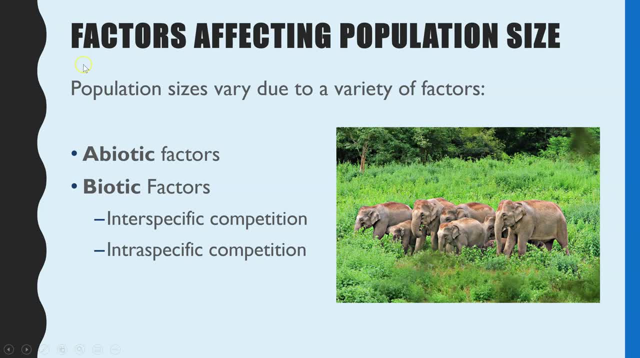 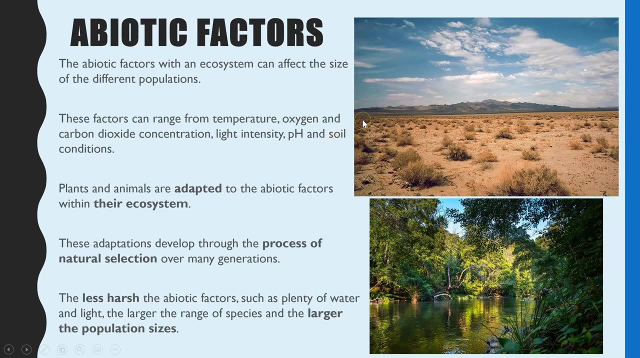 So the size of a population does vary, And that's varying depending on mainly these two factors: The abiotic factors they're exposed to and the biotic factors. And in particular we're going to be looking at competition. So first of all, then, abiotic factors. So within the definition we said that these are the non-living factors. 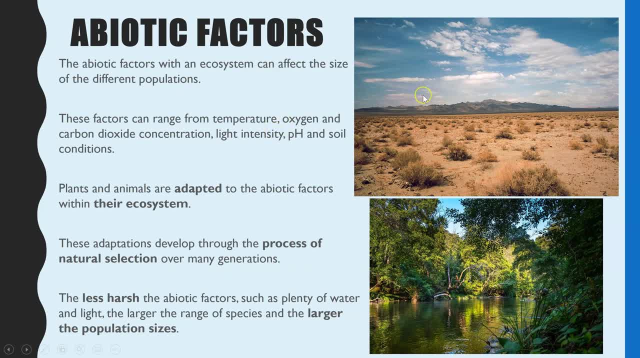 These are the non-living components of the ecosystem. So, for example, that could be the temperature and oxygen, And now that is particularly important if we are talking about an aquatic ecosystem, So the amount of oxygen dissolved in the water and the amount of carbon dioxide in the atmosphere. 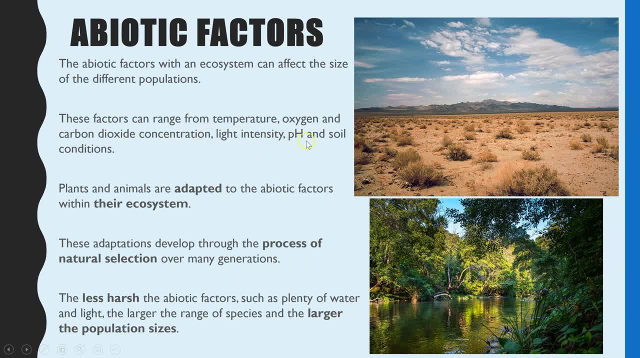 Or again, it could be dissolved in water, light intensity, pH of soil, It could be mineral content of soil. So just bear in mind That is not sufficient to say climate is an abiotic factor. You'd really need to pick out which aspect of the climate 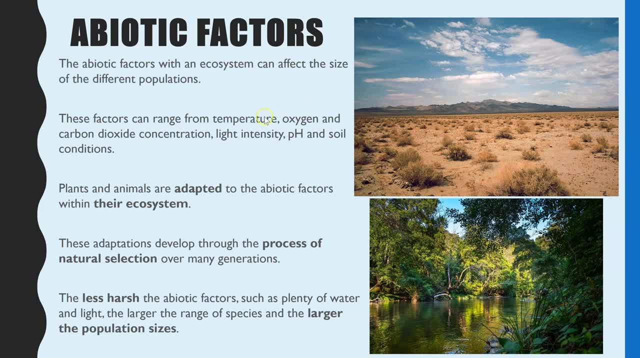 Because climate could link to the amount of precipitation, temperature, light intensity, And plants and animals are adapted to the abiotic factors within their ecosystem. So you could get some questions linked to adaptations And if you think about different plant species, adaptations to very little water content in the soil could be very, very extensive root networks. 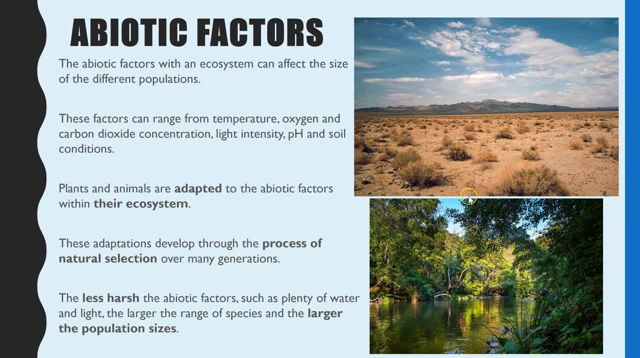 Or plants growing very broad leaves to try and get a larger surface area to obtain light. And these adaptations link to the topic of natural selection, Because it would take many, many generations before the entire species possessed that particular adaptation. The final thing, linked to abiotic factors, is the less harsh the abiotic factors. 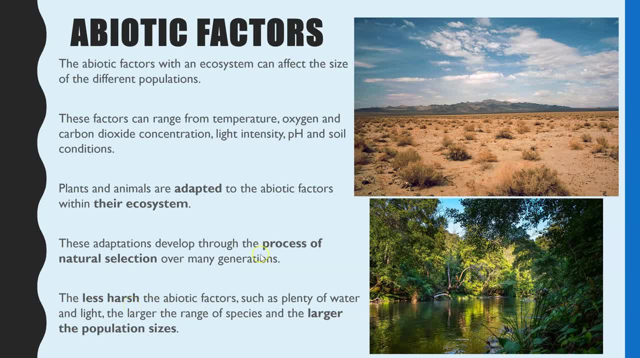 And what I mean by that is you have plenty of all the conditions you need, So it could be plenty of water, lights. That would then mean that that particular ecosystem is able to support a much larger range of species, And each species will be able to have a larger population size. 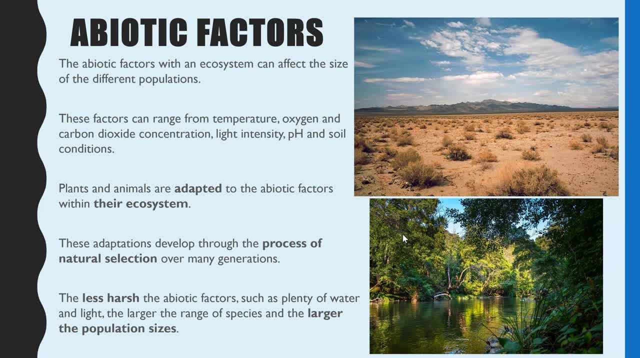 So that's why I've got these two images, Just to demonstrate that point. So we've got the bottom picture just showing that we've got plenty of water availability. We can see lots of blue sky, lots of sunshine as well. So just thinking about those two abiotic factors has enabled. 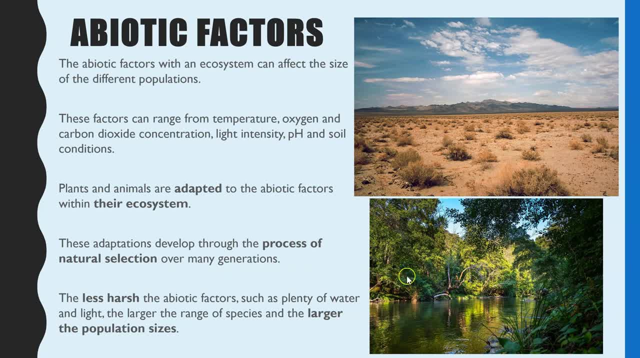 We can see a whole range of different plant species. There will be animals as well, but we can't see those in this image. There's lots of different plant species and there's lots of them, Whereas the top picture We can see far harsher abiotic factors. 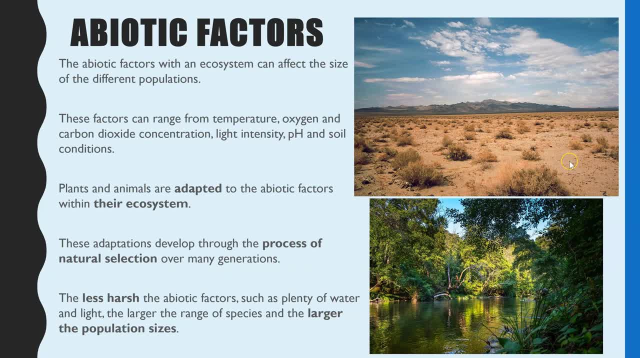 So in the desert we can see that the soil must be very low in nutrients because it looks more like sand. Very little water content. There is lots of sunlight available, But if there's not much nutrients or water in the soil that's going to make growth and photosynthesis challenging. 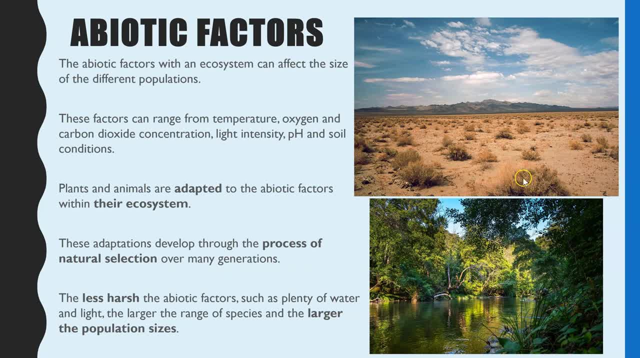 And for that reason we can see there are very, very few different plant species And in fact it looks in this image that potentially we can only see one. There won't only be one, but there's far fewer plant species and species in general. 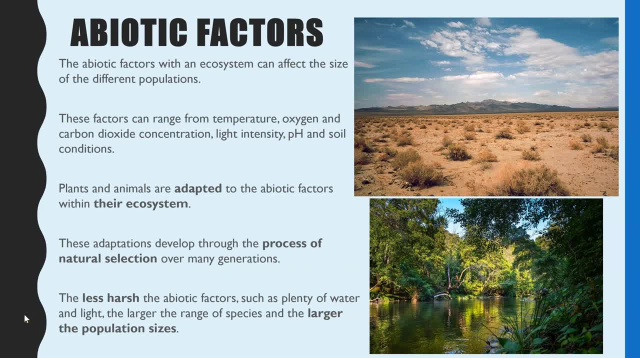 There'll be fewer animals as well, And you'll also find there are fewer individuals within each species, So the population sizes will be smaller. So that is how abiotic factors affect the population size. So the next factor to consider is biotic factors. 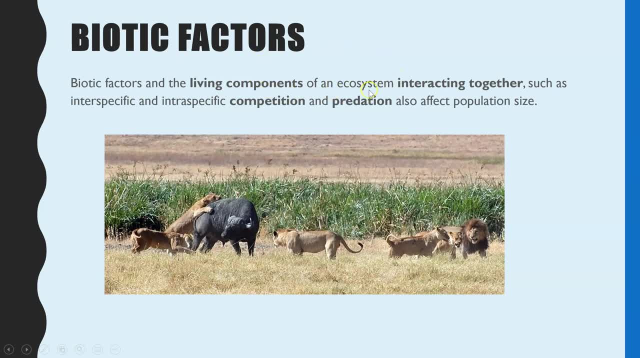 And these are the living components of an ecosystem. But it's not just thinking about living components. It's looking at how different organisms interact together, And that's where it leads us on to competition, And, in particular, we'll be looking at predation. 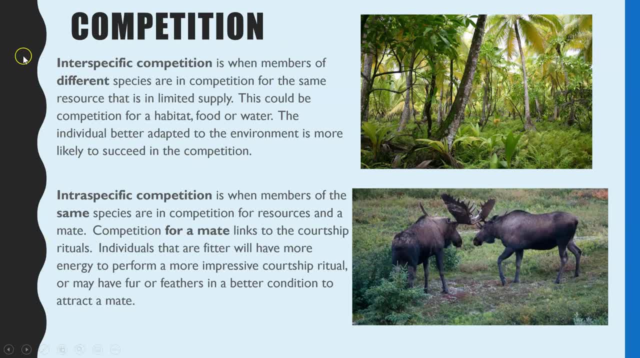 So competition? this is the same as it was at GCSE. So you have two different types of competition: Interspecific, so TER, And that is when it is organisms between different species competing. Intraspecific, so TRA, Is when members of the same species are competing. 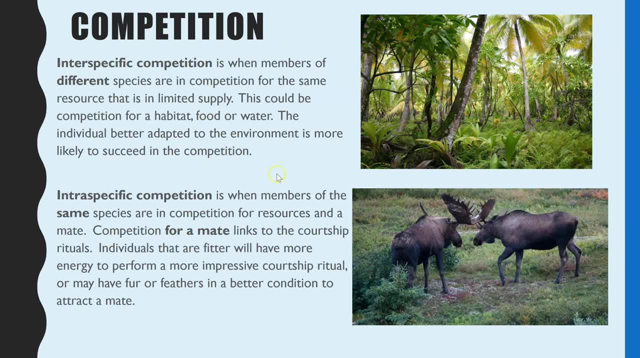 Now, in both types of competition, whether it's between the same species or different species, there will be competition for space, It could be for food, water, But the key difference is members of the same species will also be competing for mates, And that's where this then links to courtship rituals. 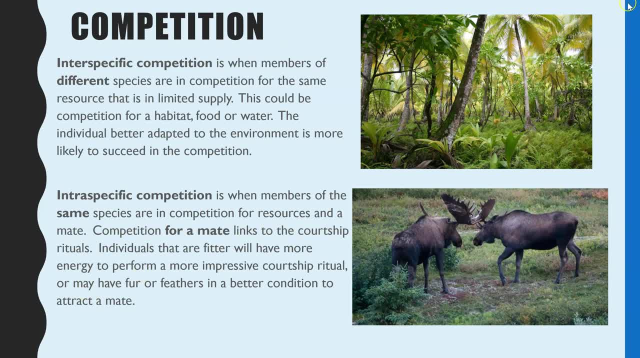 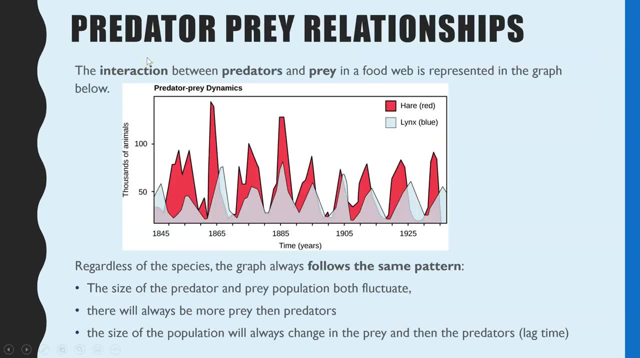 And I'll link the video for courtship rituals just up here So if you haven't seen that, you can check out courtship rituals. So that takes us on to the predator prey relationships, So the interactions between predators and prey within a particular ecosystem. 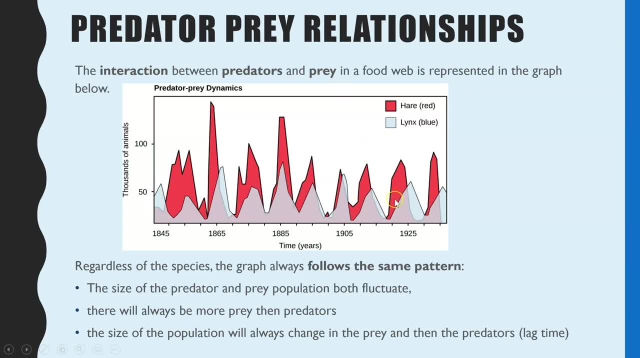 will typically follow this style graph And you could be asked to either describe or explain the patterns on a predator prey graph And what I've just done is picked out the key patterns that you will see for any species. So, although we've got hare and lynx- hare being the prey and lynx being the predator- 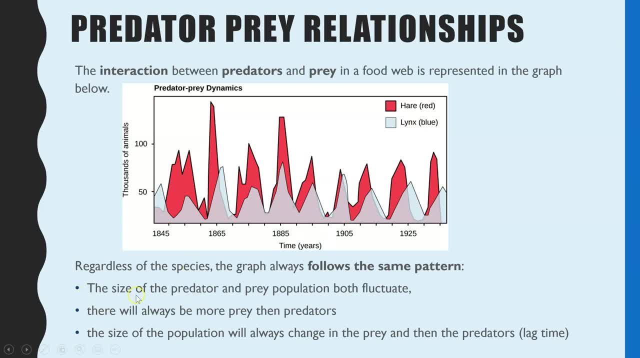 you will typically see these three patterns, whichever predator and prey you are given. So, number one, the size of the predator and the prey population both fluctuate, So that's the first thing we can see. You don't have this static population size. 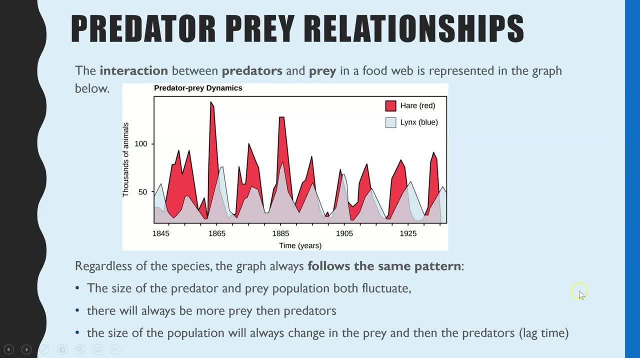 Both of them are going up and down, up and down, up and down, And that is because, as you get this increase in prey, that is then more food for the predators, So the predators get more food. That means they can reproduce more and you get more predators. 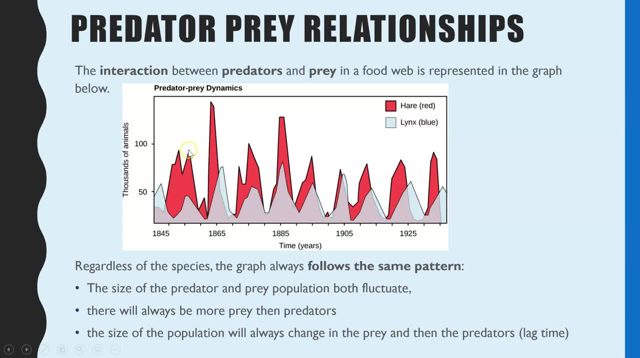 But as you get more predators, that means there's more of them to eat the prey, So the population of prey decreases. When the population of prey decreases, there's then not enough food for the predators, So they start to die out. And again you just get this pattern happening on loop. 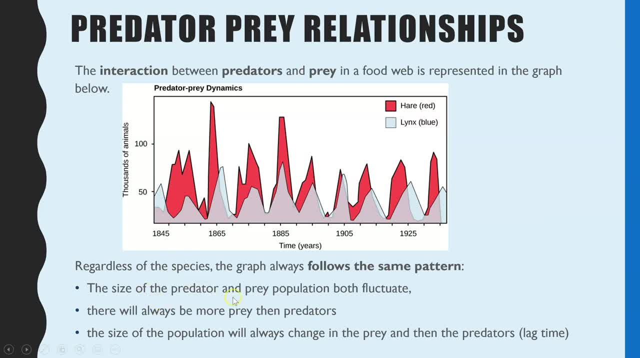 Over and, over and over. So that is the first pattern: There will always be more prey than predators. Now, for that one, I'm just going to tweak that slightly, to say- the prey population will always peak at a higher point, Because you might sometimes see that occasionally there are more predators than prey. 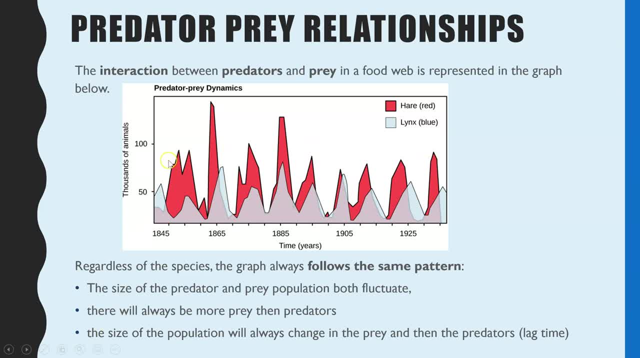 But overall you tend to have more prey than predators, And the prey peak in population size is always higher And that's because the predators are further along the food chain And that means whatever they are eating will contain less energy, Because energy is wasted at every trophic level. 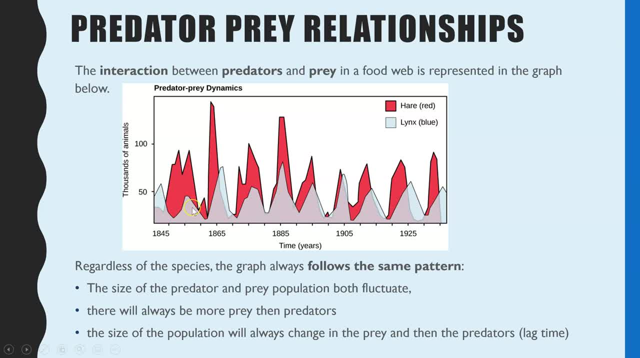 So in order for them to gain enough energy from their food, they have to eat more of that particular animal. So to be able to sustain one lynx they will need to be eating multiple prey. So you won't typically see more predators than the food source, the prey. for that reason, 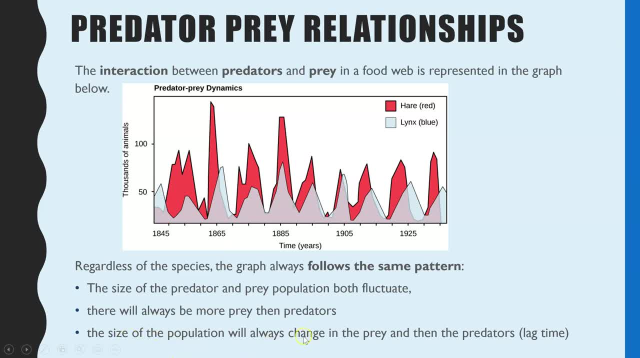 The last pattern is the size of the population will always change in the prey first, And then there's this lag time before the predator population changes And that's what we can see quite clearly in 1845.. We have this increase in the prey population. 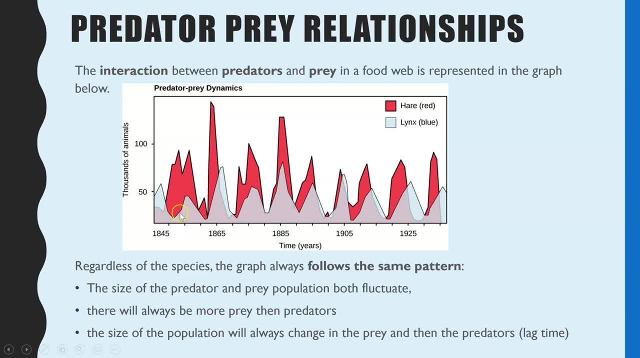 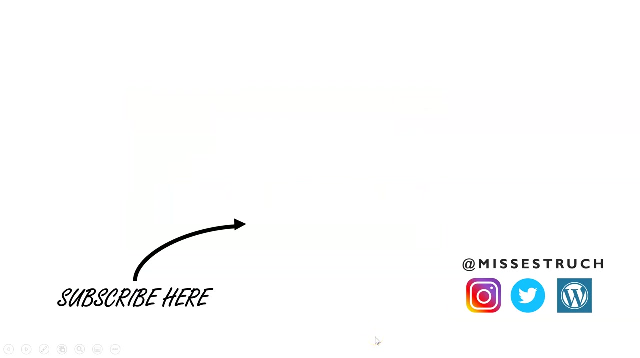 And then it's not until a year or so later that you start to see the increase in the predator population. Then the prey population decreases first, And then the predator population decreases, So you get this lag time as well. So that is it for the abiotic and biotic factors.